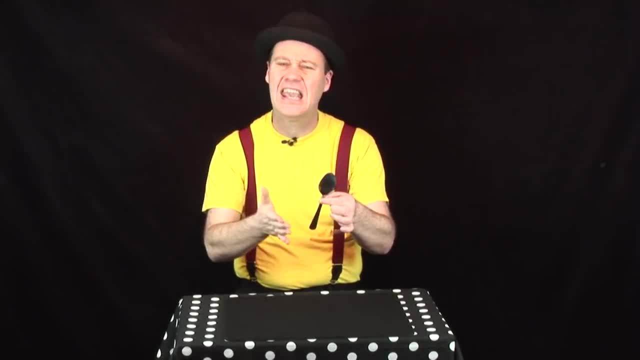 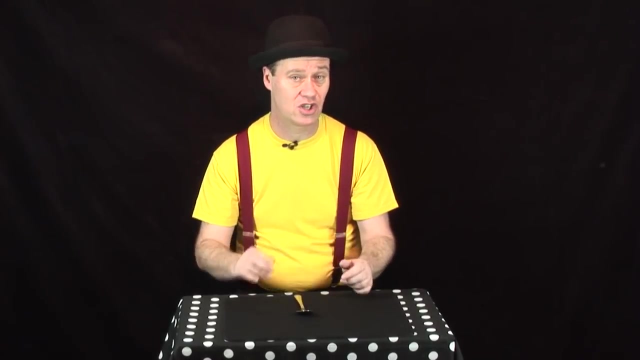 Uri Geller was really famous for bending keys and bending spoons and bending forks, and I'm going to show you how you can bend any spoon in any restaurant that you go to. Now, this is a lot of fun and the cool thing is you don't need any special equipment, you just need to watch closely. 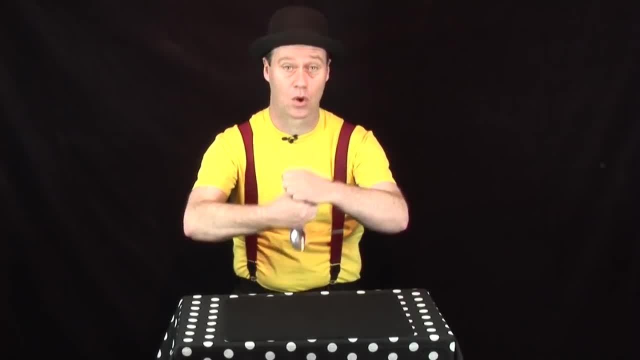 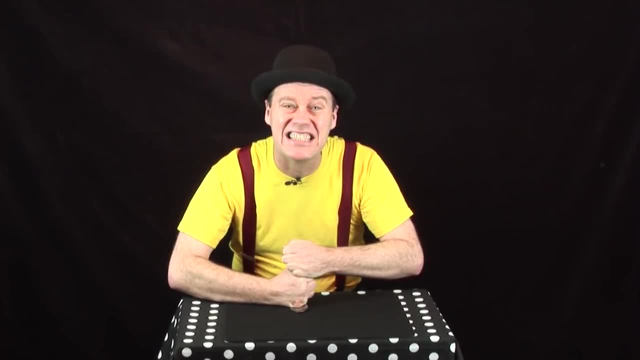 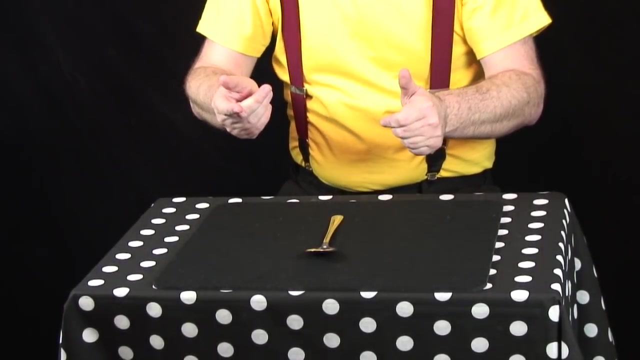 We're going to take the spoon, going to hold it nice and tight. watch this. It's definitely bent. Now that doesn't look too impressive, does it? But what is impressive is how we just go back in time and get a bent spoon back to a straight spoon by magic. Believe me. 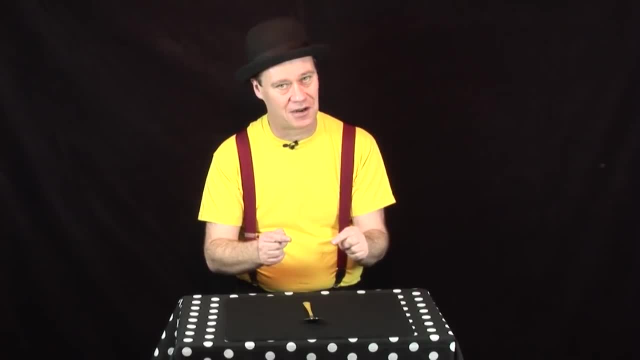 if you do this in a restaurant, at a table, every eye is going to be on you. They're going to wonder how you did it, and I'm going to show you how you can do it, because you can do magic. Look at that. it looks just. 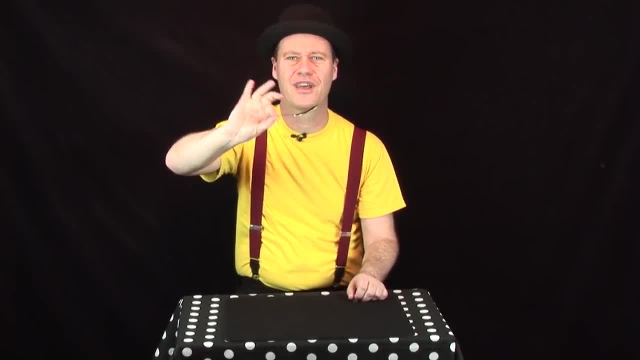 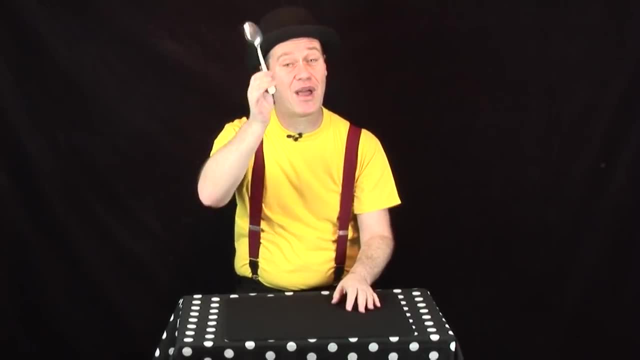 like a rubber spoon. You can do this with anything. you can do it with the fork, you can do with a pencil. if you just kind of hold it and give it a wiggle like that, and it almost looks like it's bending, doesn't it? It almost looks really weird. but this just is a regular spoon and I'm going. 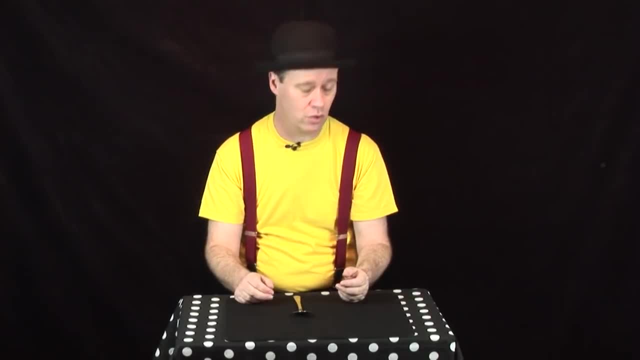 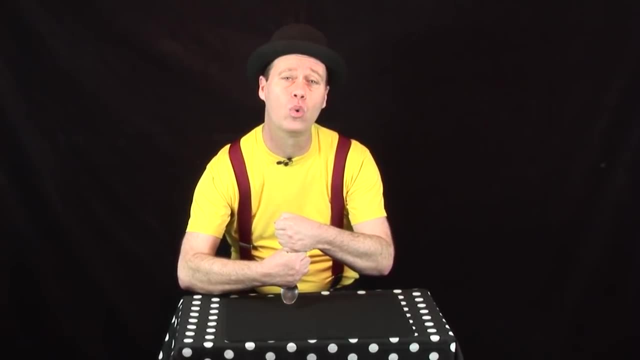 to show you how I did that bend and that restore of the spoon so that you can do it. Yep, it's all to do with the way that you hold the spoon. So it looks from the front like I'm holding thatgamma5 achoey. There you have it、 bent, and how it looks from the front. 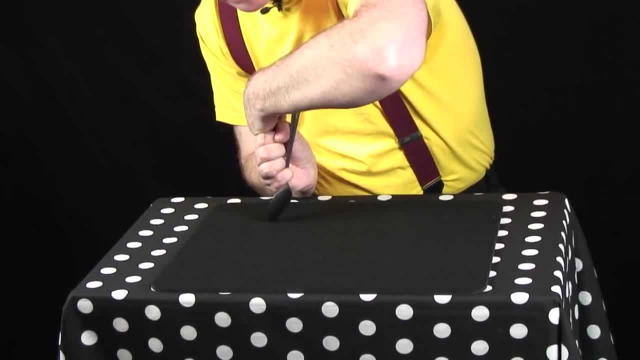 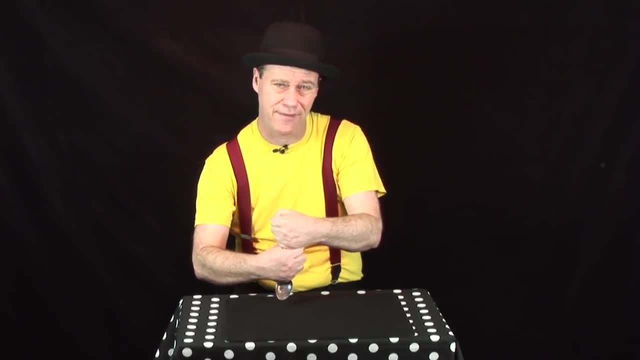 spoon correctly. but if you could see from the back, you would notice that i'm actually not holding the spoon. all i'm doing is holding it with one finger. now, if you want to see this exact grip- it's pretty difficult for me to turn all the way around to show you- just head on over to our website. it's. 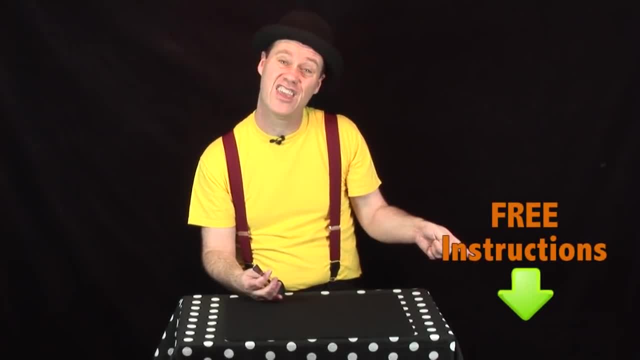 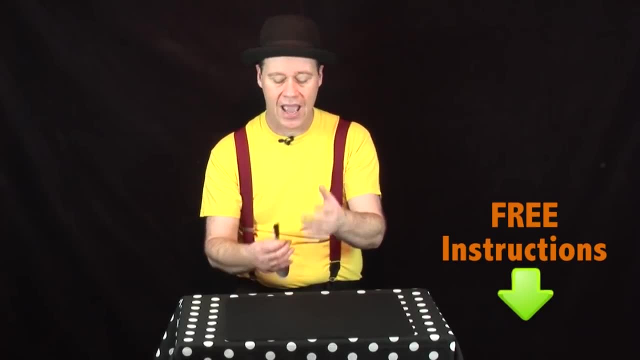 magictricksforkidsorg. there's the link right over there. you can just click on it. that'll take you through and it's got photographs showing you the back of this. it's free. you can download it if you like, yeah, and you can learn how to do this, but i'll show you the handling. so you're holding the. 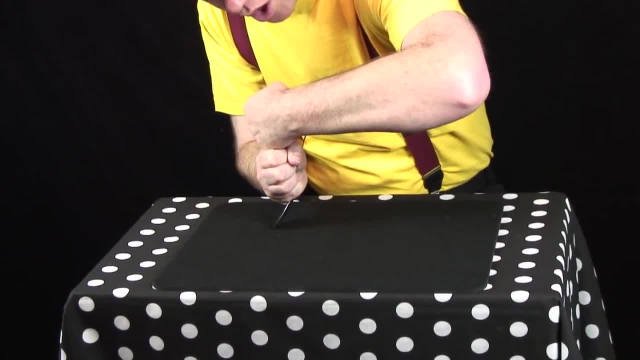 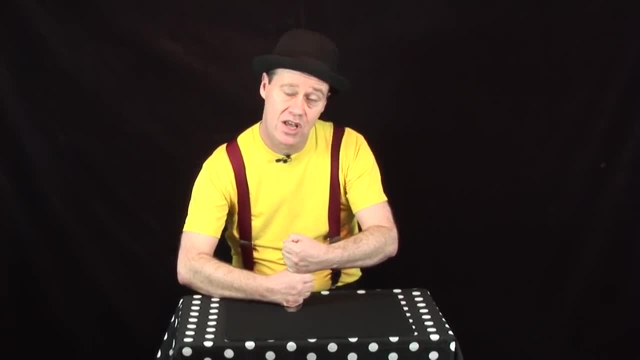 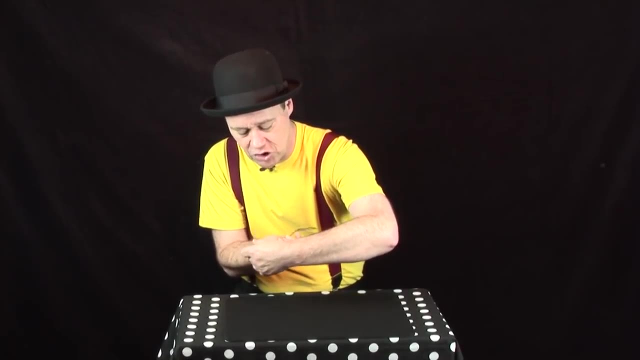 spoon in that special grip. as you push down, what's happening is the spoon is just going down behind your hands. from the front really looks like that spoon has been bent, and then to restore it you just lift it back up again, close your pinky, which is actually holding that spoon, and then turn the